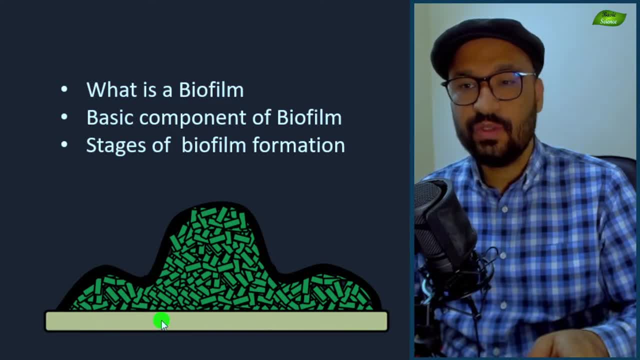 In this case, as you can see here in yellow color, I have shown a substrate. Now you will see another layer which is on the top of the bacterial growth, And that's the protective layer. Bacteria also have this layer so that cells can be protected. It is like we have houses. we have buildings. 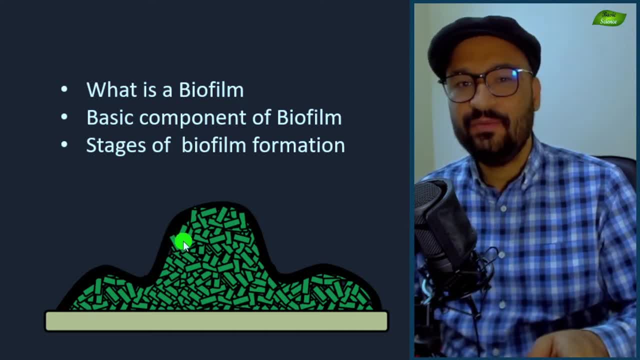 and we are protected by those buildings And we live inside those buildings. In a similar way, bacteria also have a protective layer, So that cells can be protected. In a similar way, bacteria can also live inside these communities as a communities, inside these structures. 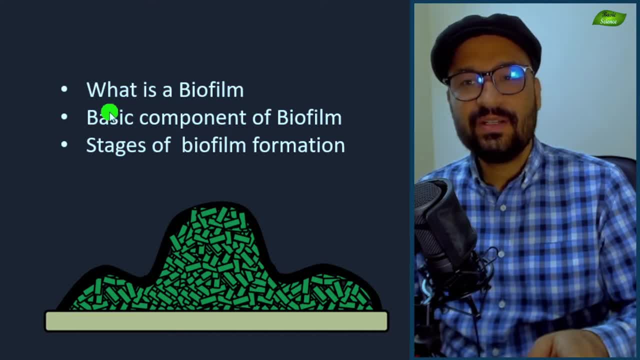 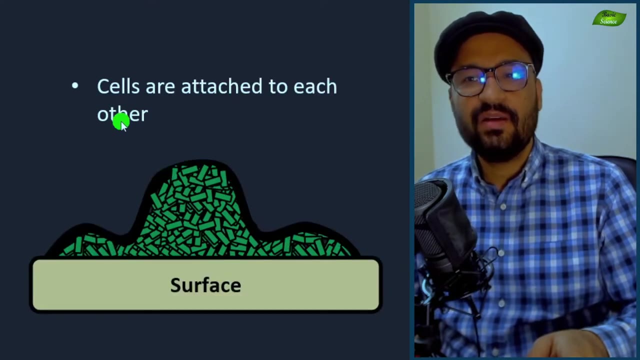 Bacterial Biofilm Structure. So hopefully you will be able to understand what is a bacterial biofilm. I'll discuss small stages of biofilm formation- Bacterial Biofilm Structure. So let's go on to the next slide. Here, what I am trying to show you is bacterial biofilm is not just the attachment to the surface. Bacterial Biofilm: Structure, shape of the site. Here, what I am trying to show you is bacterial biofilm is not just the attachment to the surface. This is basically what we have showed you is the muchísimo formation of biofilm. 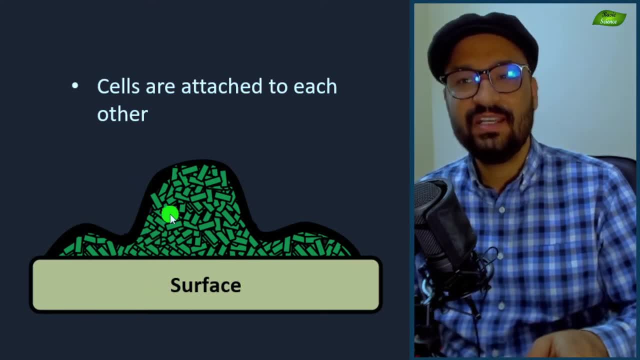 the angulation, the dermo, the reconstrible związ thứ occurring within the skin of the Finnish, the cells. they are also attached to each other, so they will start attaching to the surface, they will start adhering together. then they will start secreting various complex structures. they will 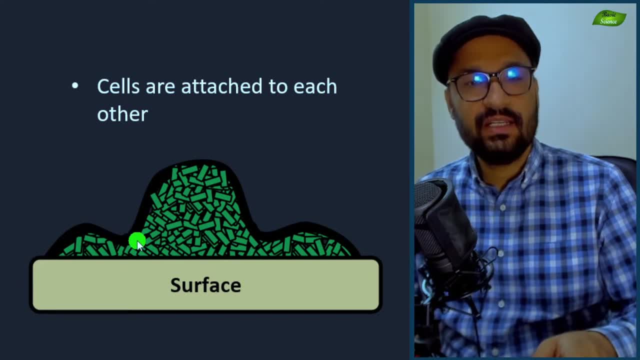 start secreting proteins. they will start screening lipo polysaccharides and just lipids. they will start secreting polysaccharides, they will start secreting DNA and that, will you know, work as the architecture that will help to build that architecture and slowly, slowly, then bacteria. 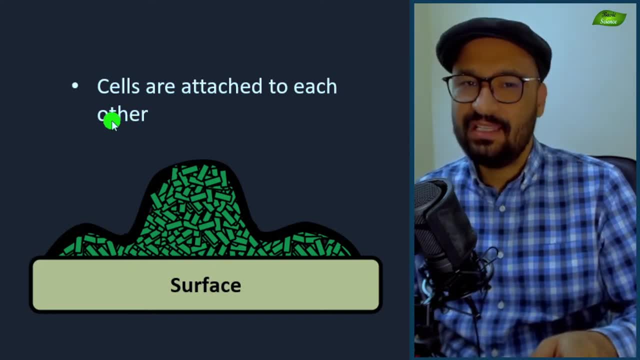 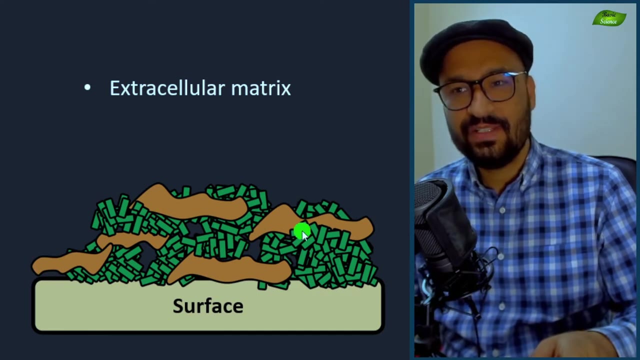 is going to build a three-dimensional structure which is the biofilm and biofilms. they are highly, highly important in in many scenarios. so we'll discuss all those cases now. let's move on to the another slide, and you can see here I have another structure which is shown in orange color and this: 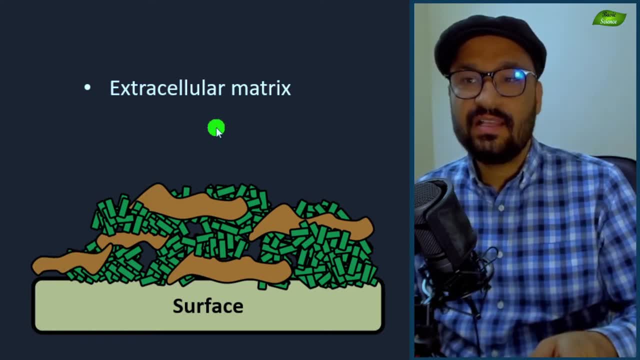 I want to show is the extracellular matrix. apart from the cell, bacterial cells, they are going to secrete a specific type of matrix which is composed of polysaccharides, which will be composed of, as I have already mentioned, proteins and some other chemical compounds, and that will help the 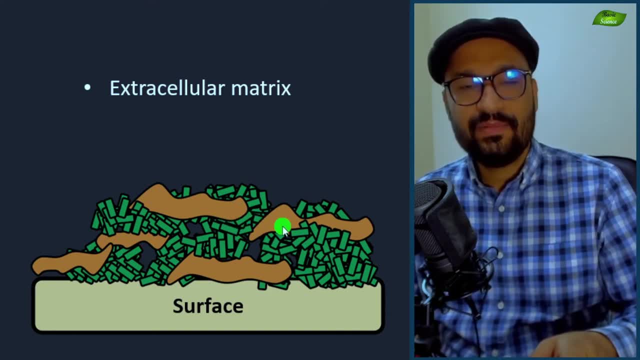 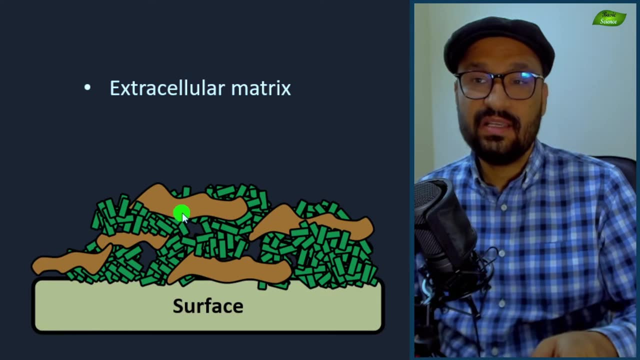 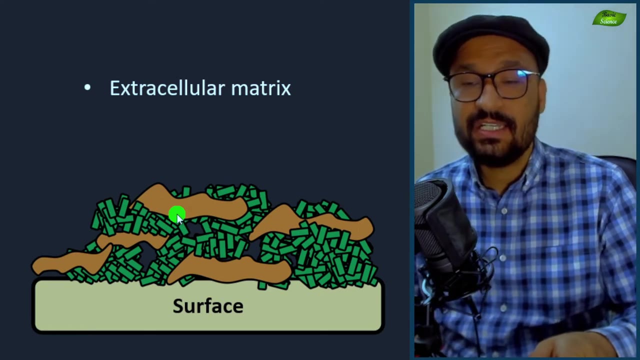 integrity of the biofilm. that will help in the structure of the biofilm and it is very, very important. and because of this extracellular matrix bacteria, they are protected from environmental factors. they are protected from antimicrobial agents or some other chemical compounds. so, as you can see, here you have the 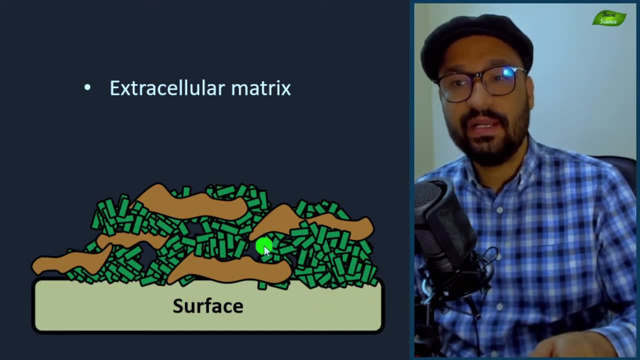 surface, on déc, on the top of that surface you have bacterial cells and they are attached first on the surface and they are also attached to the cellический无ιλ and they are also attached in this way together, and then they have this extracellular matrix, which is highly, highly complex, and then 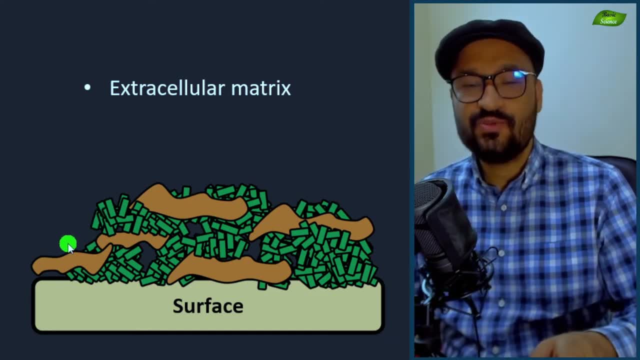 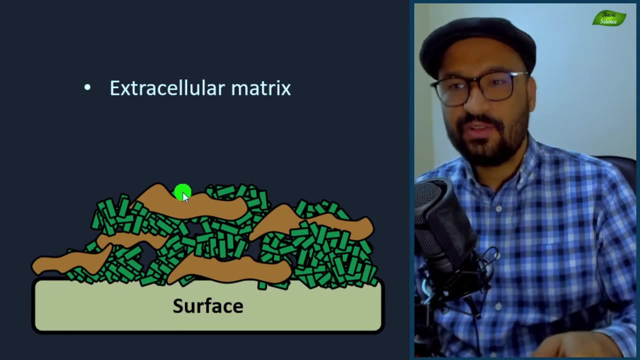 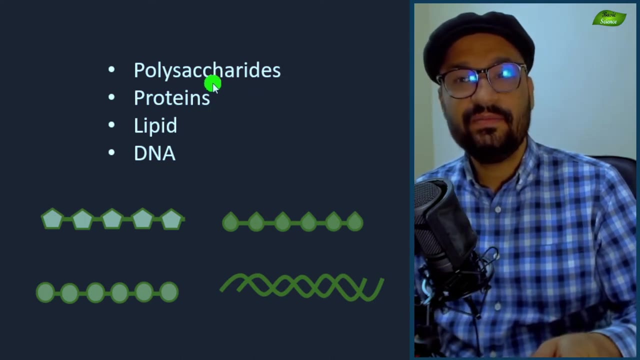 you will construct, or bacteria is going to construct, a lot of different three-dimensional structure. so that is your biofilm and this is the basic structure of the biofilm. now, what is the? what are the different components inside the biofilms? you have polysaccharides that i have. 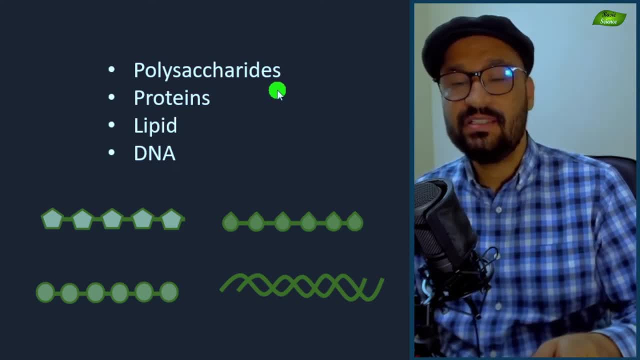 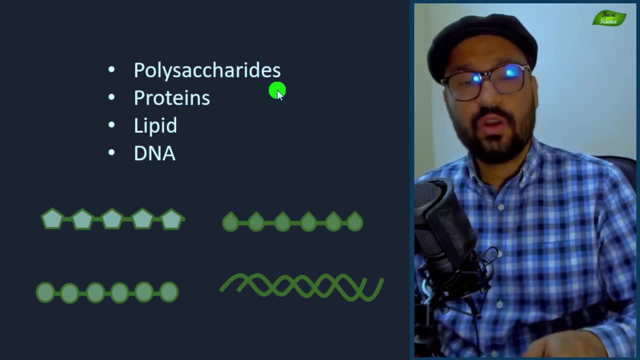 already told you that there will be different types of polysaccharides depending upon the biofilm. first, you need to remember that when we talk about biofilms in nature, we are not going to have a single organism. we'll have multiple types of organisms and they are constantly interacting. 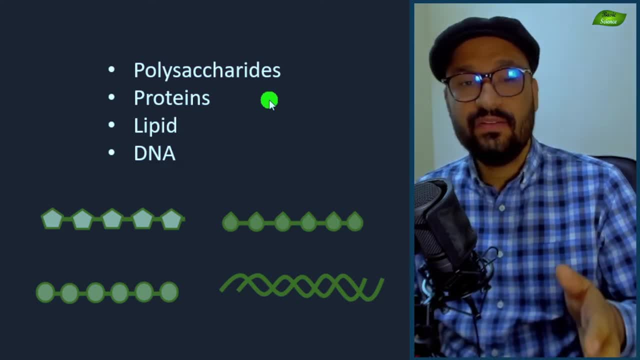 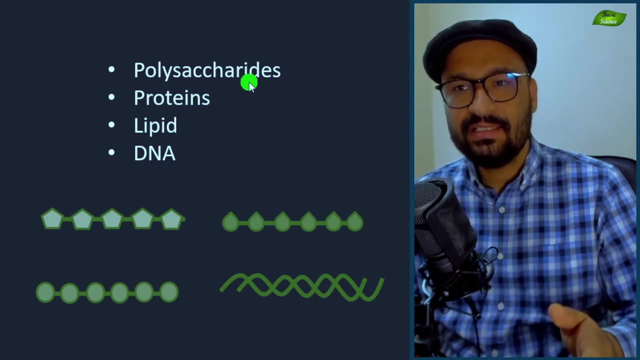 with each other. some organisms, they will try to inhibit the other organism. some organisms, they will try to promote the growth of one organism. so it will be a dynamic process, you and then they will start secreting various components like polysaccharides, which is basically the chain of saccharide molecules, the chain of. you know, that's why you say chain of. 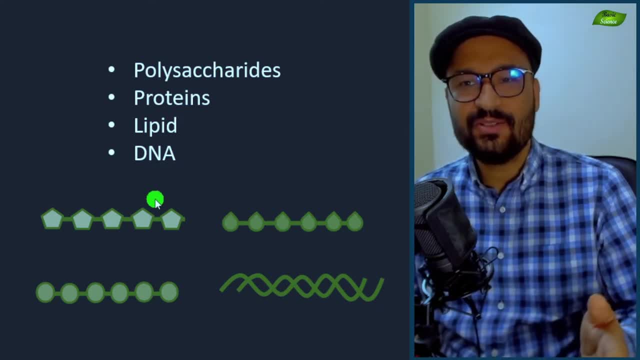 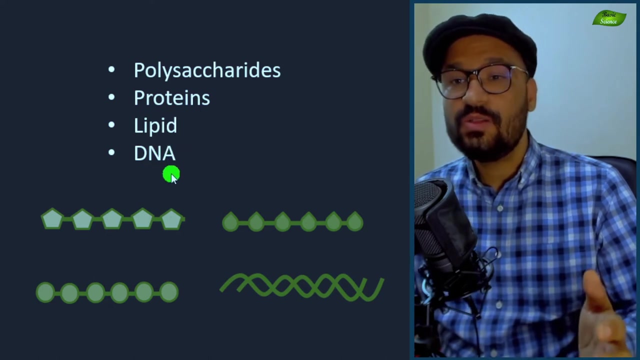 sugar molecules. poly means a lot of sugar molecules- and then you'll have proteins, and we also know that protein is basically the chain of amino acids, so it's a biopolymer molecule. then you will have lipid molecules and extracellular dna. extracellular dna is also very, very important in this case, in especially in case of biofilm formation. 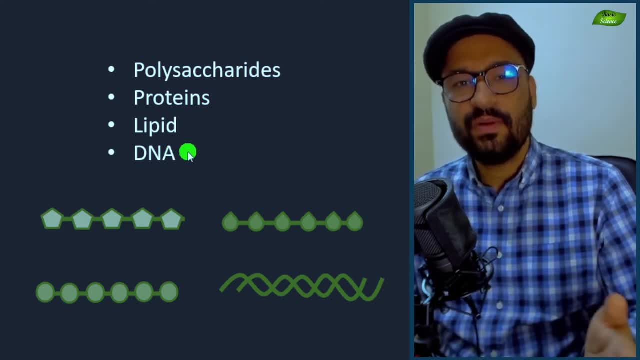 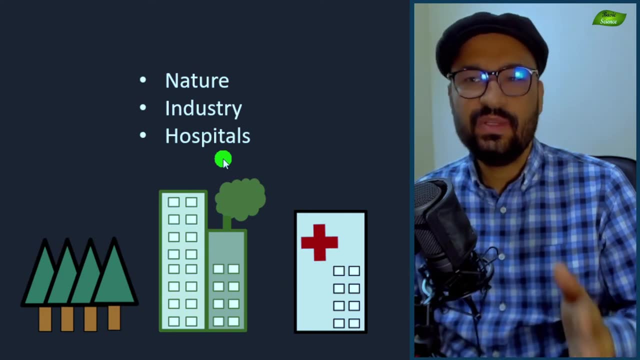 now these are the some of the basic component of the components of the biofilm. now let's move on to the final slide. so as i've already told you that in this video i'll just explain the basics. so biofilms: they are important in case of nature because in nature you have complex interaction. 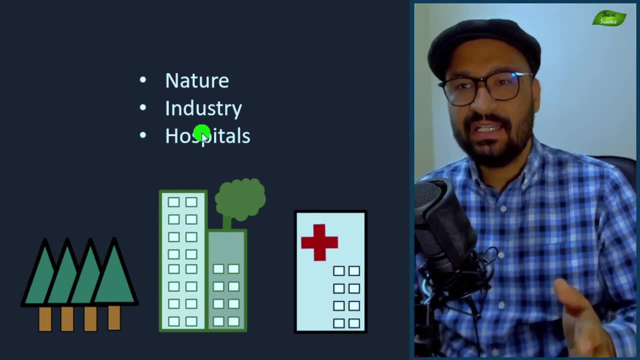 and in biofilm the same thing is happening. it's like a small, tiny ecosystem where you have different types of microorganisms living together, and when we talk about bacterial biofilm, i'm just talking about the biofilm of the bacteria, but you'll have various types of organisms in the biofilm that are present in nature. second industry, so in industry. 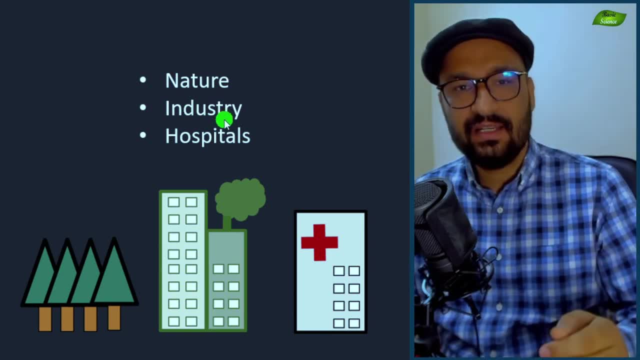 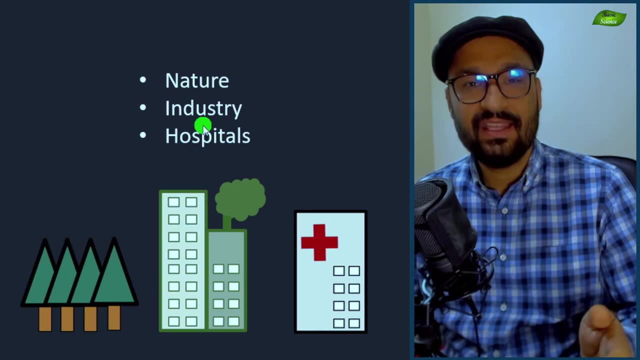 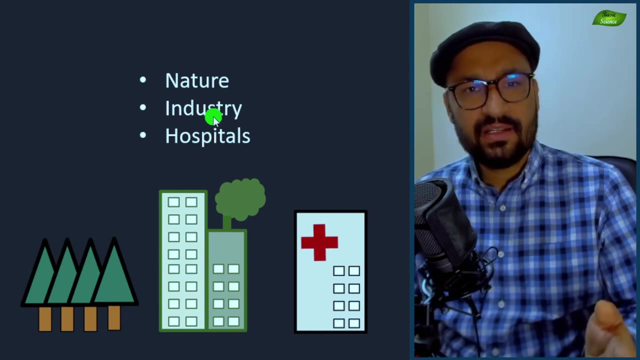 you have lot of different types of industries right and where, especially the food industry, where the environment is nutritious for organisms- bacteria- they are going to grow and biofilm is going to get formed because of that nutrition. and then in chemical industry you'll find bacterial biophilms over there as well. hospitals in hospitals. 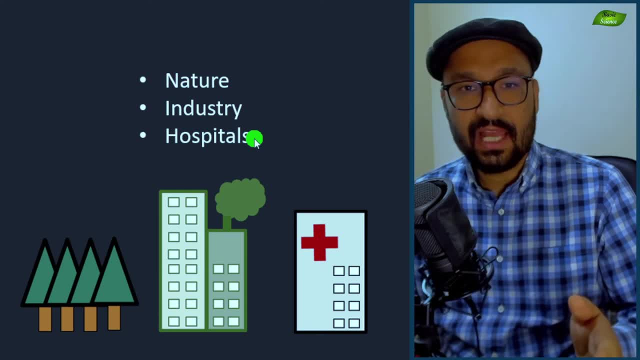 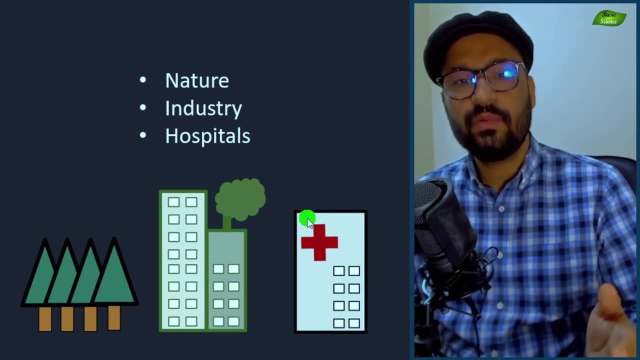 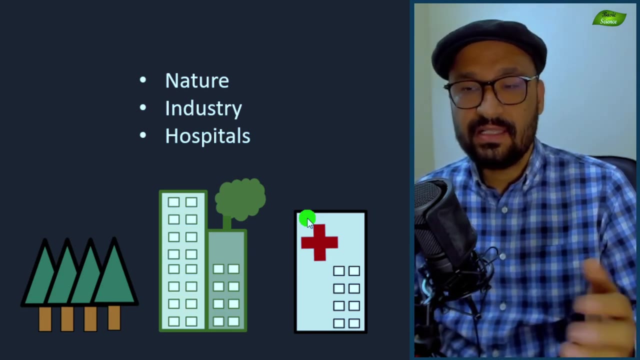 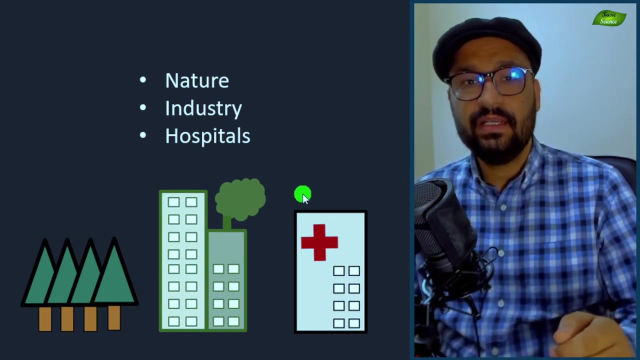 bacterial biofilm formation is a huge challenge because if bacteria is going to form biofilm in environment like hospital, then they are going to get protected by various agents which are antiseptic agents and then they are going to form the resistance against these specifically antivacuable resistance against antibiotics, because in hospital you will find 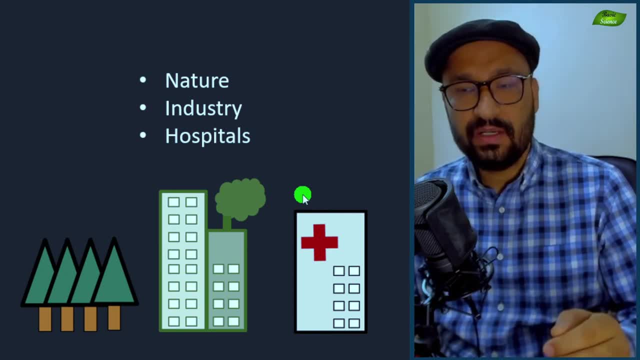 various kind of chemical treatments for the sanitization. if the bacteria is growing in that condition, that means the bacteria is really resistant. and also it's important because then you have immunocompromised patients in hospitals and they are prone to infection. so this is, this is